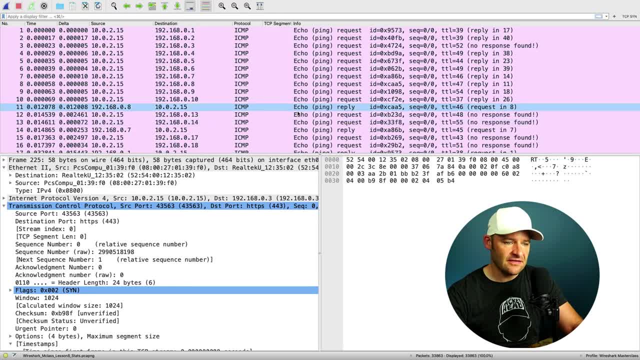 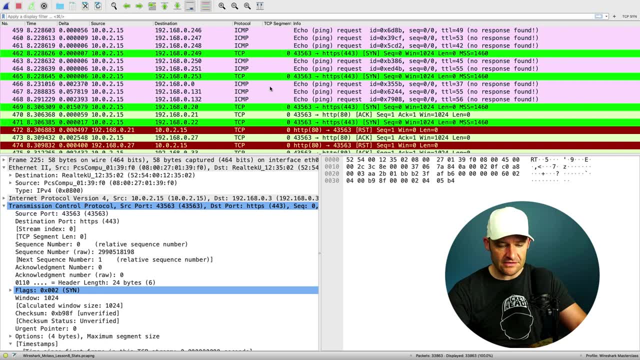 Okay, so let's go ahead and get to the PCAP. So here right away, we can see that we have some pings going on. If I really scroll down below that, I got some TCP sends. I got some things going on in this trace file. If I take a glance down at the number of packets that I have, I got 33.. 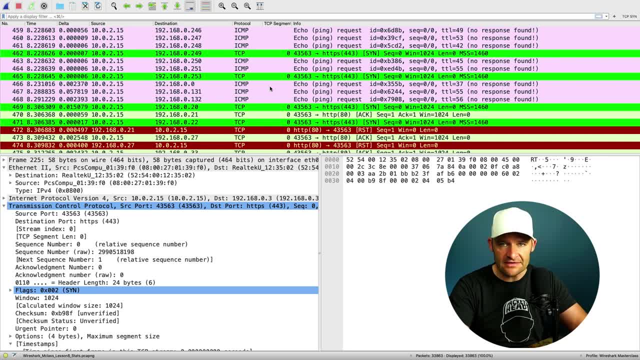 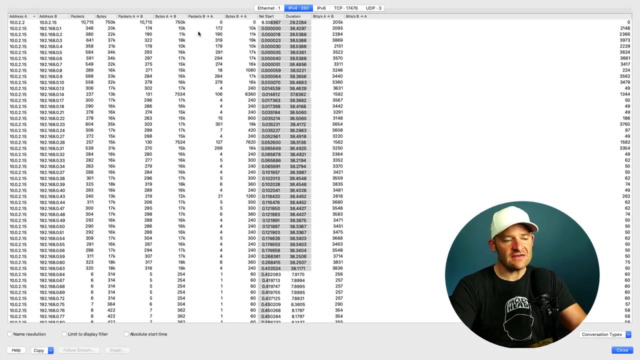 1,863 packets in this trace And, of course, not really sure exactly what I'm looking at just yet, unless I was actually the one to capture this traffic. So I almost do this like muscle memory every single time that I open up a PCAP And that is come up to the statistics menu And what I like to do is come down to conversations. All right, So what conversations will do is it will show me, by layer of address, how many conversations that I have. 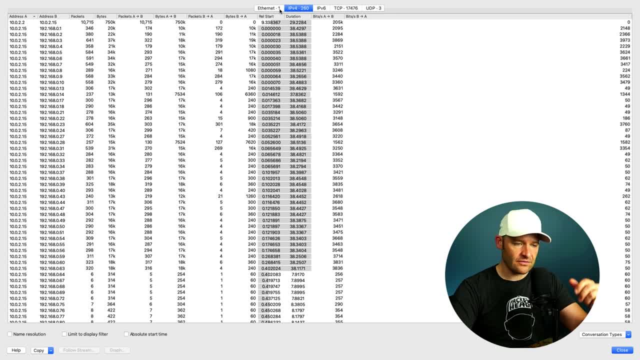 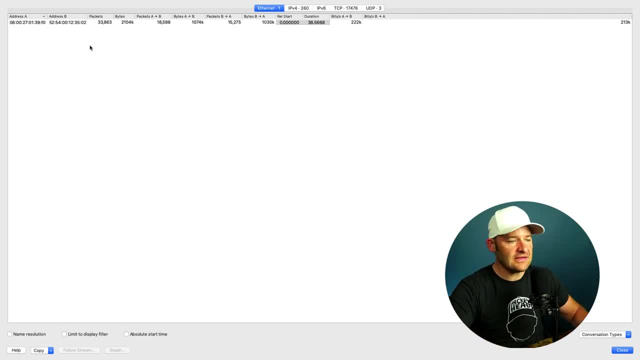 that I have in this trace file. So let me show you what I mean. Ethernet, for example. Well, I only have two MAC addresses at layer two that are talking to one another And quickly, by looking at the bytes and looking at the packets, I can see that these two are having a conversation back. 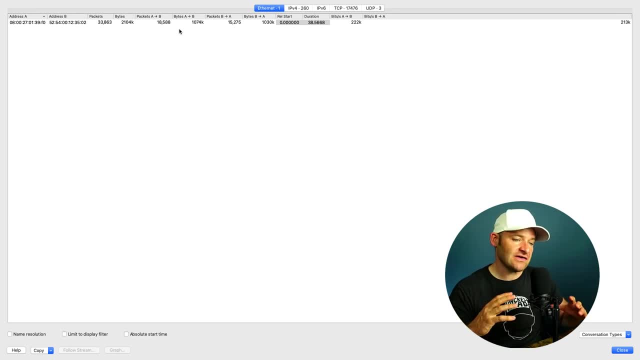 and forth. Now it could be that this is one machine talking to its gateway and it's actually talking to other stations behind that gateway, But in the context of layer two, I only have one conversation. Okay, That's just good information for me to know If I come over here to IPv4,. 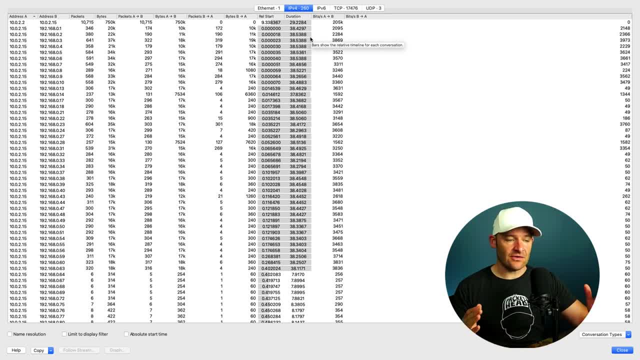 I've got 260 conversations, Whoa, a whole lot more going on. So if I come over here I can see address A, address B, the number of packets, the number of bytes, how many went from A to B? 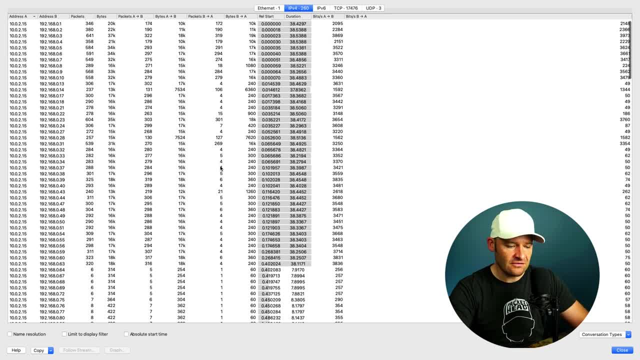 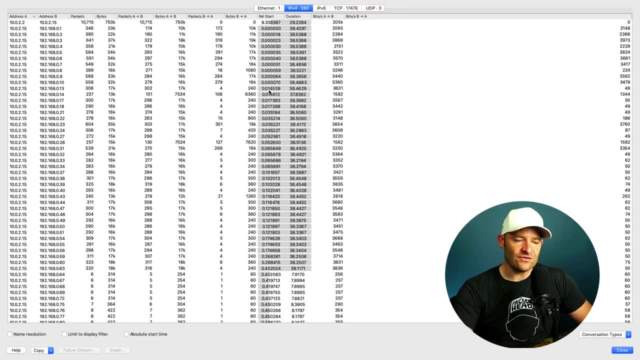 how many went from B to A and so on, And just scrolling down I can see I have quite a few that are happening. In fact, if I come over here, I like to use these two columns here as well, And this is called relative start. 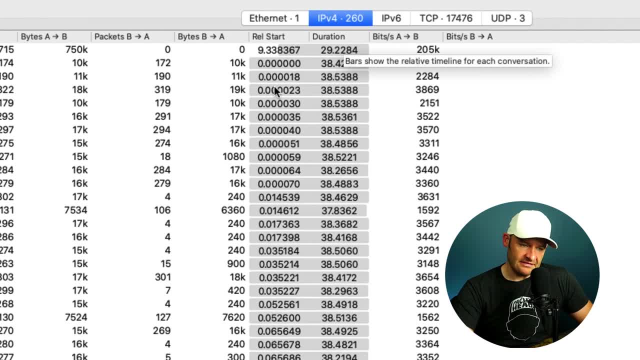 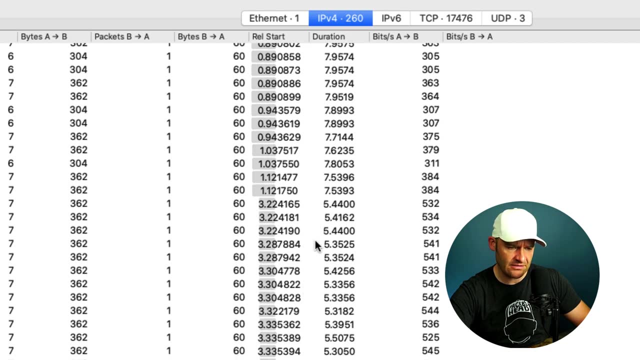 So relative start is when you're using the trace file, but you can also use relative start and duration. So the way we read this is: see, I got this gray bar here and this gives me a visual of how long lived was this conversation and where in the trace file did it start. So let me actually 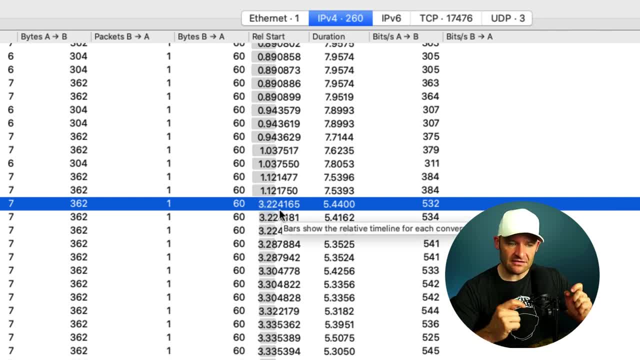 give you a better example here. I'm just going to scroll down. How about down here? So here I can see that this conversation started 3.224 seconds into the trace file and it lasted for 5.4 seconds. All right, So my first step is going to be to get it back here. So I'm going to be looking at my 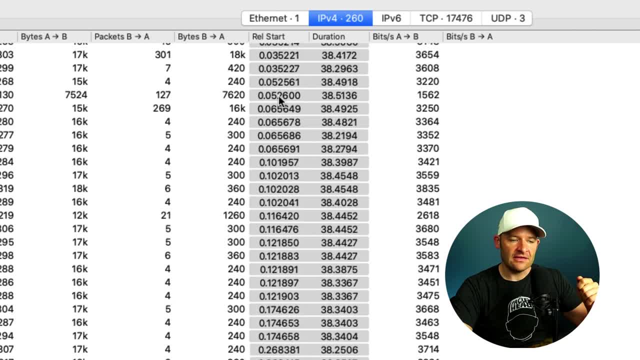 All right, so that'll help us upstairs when we see some of these longer ones. So this one happened almost exactly at the start, very close to the start, and it lasted for 38 seconds. So you see how that graphical view helps me out. 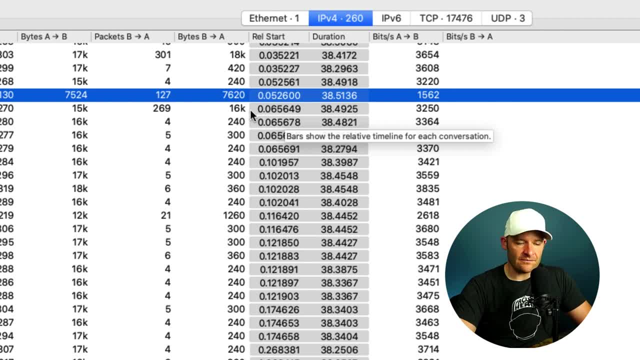 So it's the left edge of the relative start column all the way to the right edge of the duration column. That's where you'll see that graphical representation Again: it's how long lived was the conversation and when did it start, with reference from start to finish of the entire trace file. 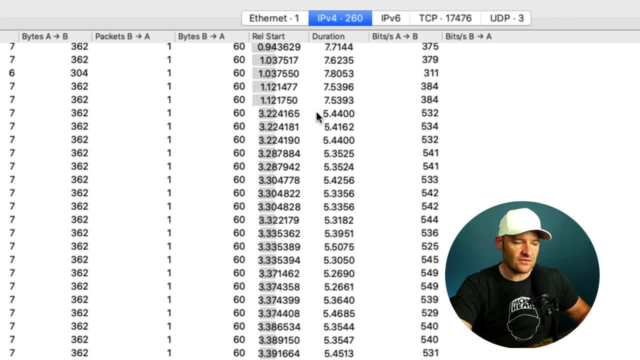 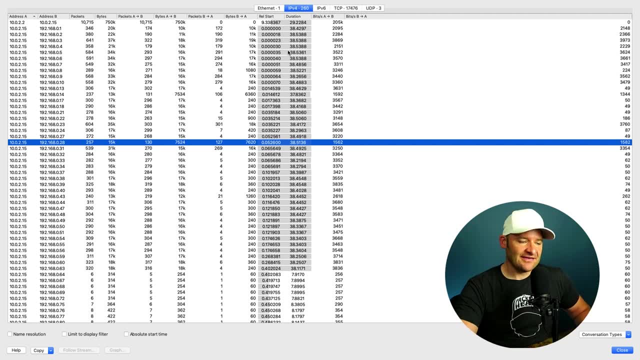 All right, so that can give me just a visual of what's going on Now. I can see right away- it doesn't take a capture guru to see- that there is some interesting things happening in this trace file If we take a look here. I've got just the link partners, if you will- the number of conversations that are happening. 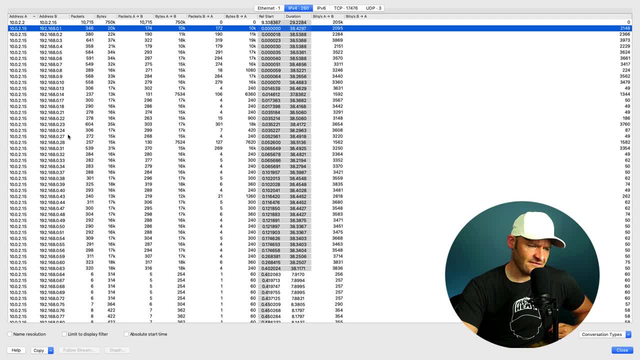 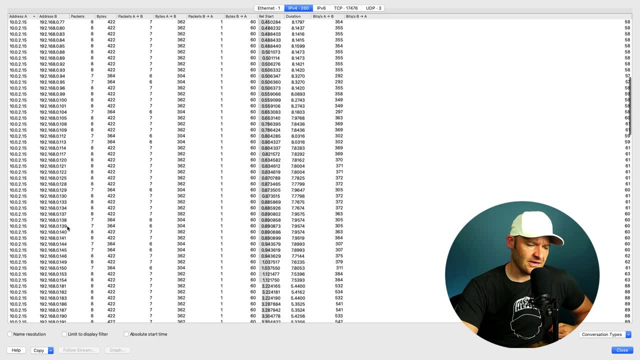 I'm looking at 0.1, 0.2, 0.3, 0.4, 0.5.. It seems almost like I'm scanning through all of these IPs, doesn't it? It seems like there's something going on here and it's happening to almost the entire subnet. 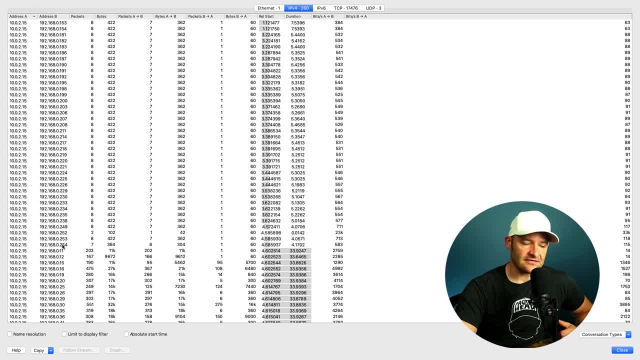 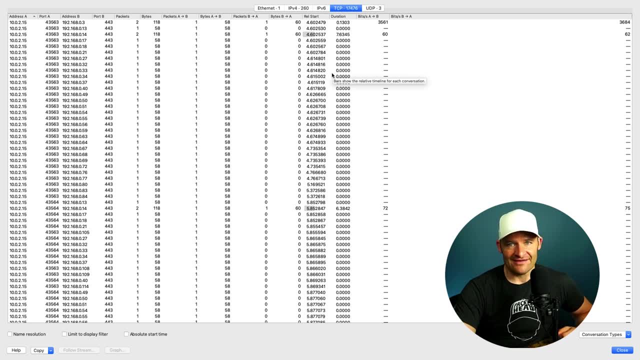 So that's something that would definitely catch my attention if I was doing some analysis here. And in fact, let's go ahead and go over to TCP. So first of all TCP: I've got 17,476 conversations. That's a ton of TCP conversations. 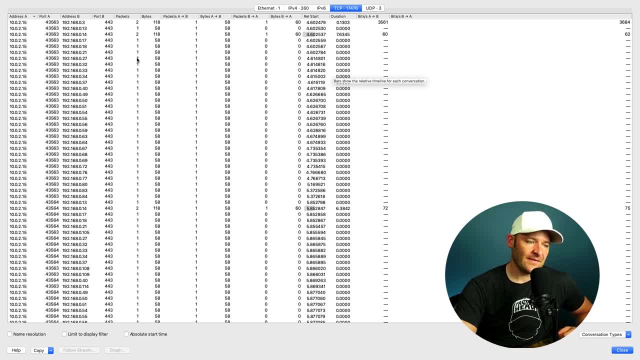 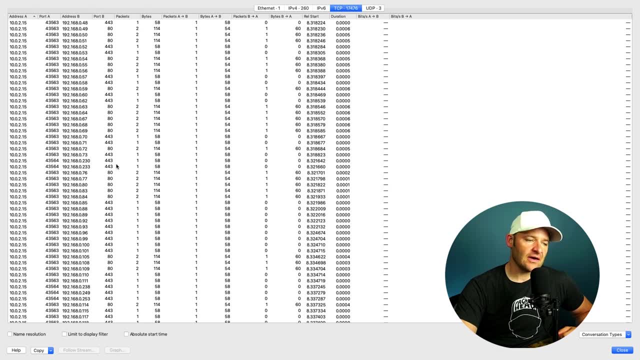 And if I look in here, you notice how the number of packets- number of packets total in these conversations- is either one or in a lot of cases I can see two or three. So that's a very low number and I can also take a look at those ports. 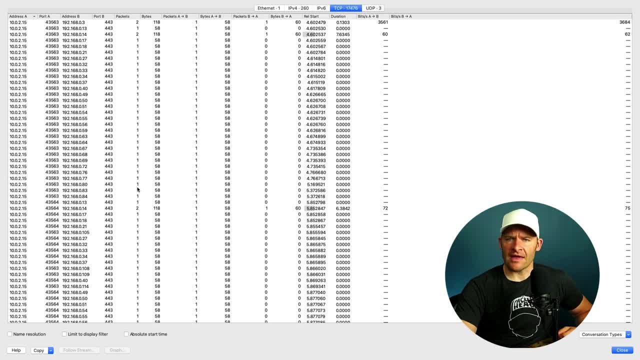 So here I can see that this is behaving really like a port scan. It's like one machine is just blasting through port 443 in the entire subnet trying to see if anybody is listening to that port. In fact, if I sort on the port B, I can see that the scanner 2.15, or 2.15, it's going out and it's hitting port one. 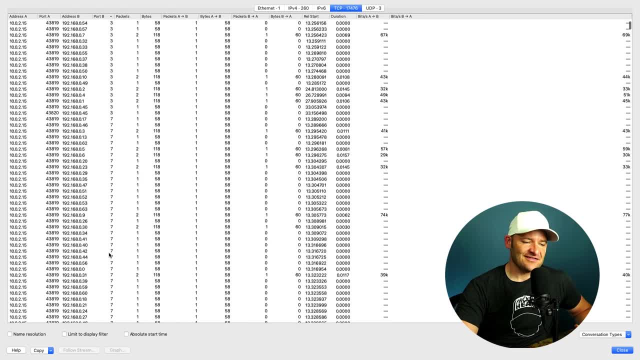 And then I can see it jump to port three, And then I can see it jump to port three, And then I can see it jump to port seven. So you see, it's not doing it sequentially: one, two, three, four, five, six, seven. 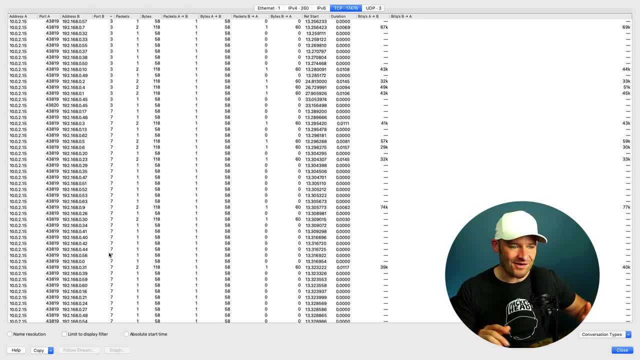 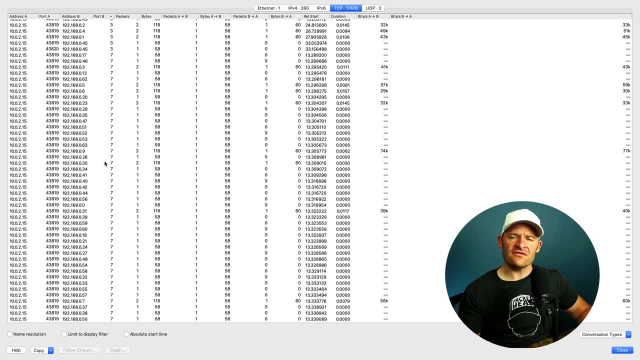 Maybe it's trying to avoid detection or do so under the radar, But I can see that this is very low port number to be trying to initiate to another device. It's very rare that I would try to hit something on port three, right. 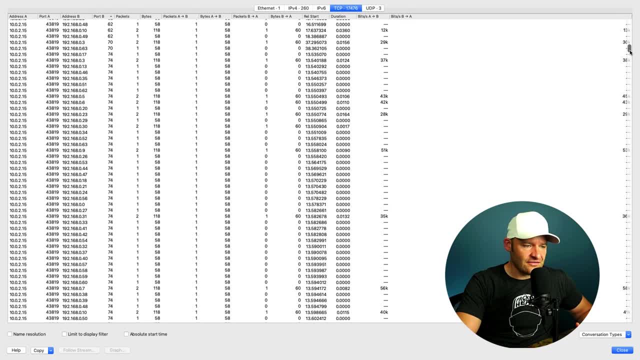 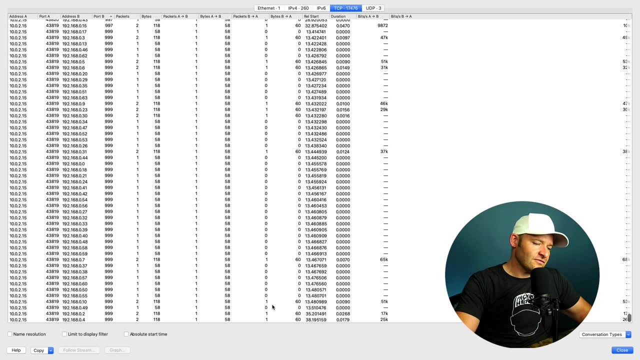 And as I scroll through here, I can see that these numbers just gradually tick up Again. they're not sequential, Looks like this scanner was trying to evade detection, And it goes all the way up to 999 on the port numbers. So just with using statistics here, I can see that this is some very unusual activity. 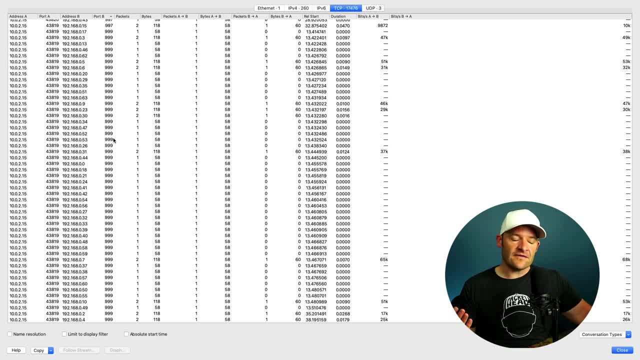 So, especially if I'm doing any type of network forensics, if I'm trying to find someone that's enumerating different devices for cybersecurity reasons, I want to check to see do I have any type of intrusions going on. There definitely would be some indicators here that I'd want to focus more attention on. 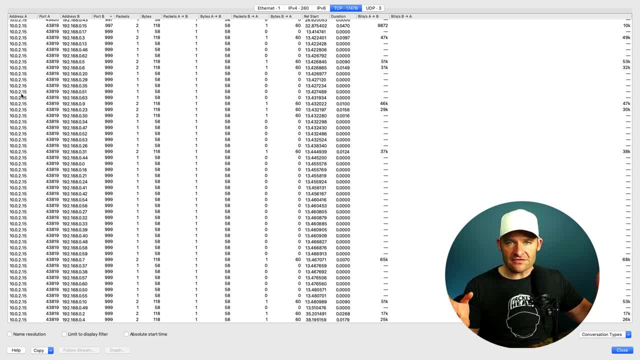 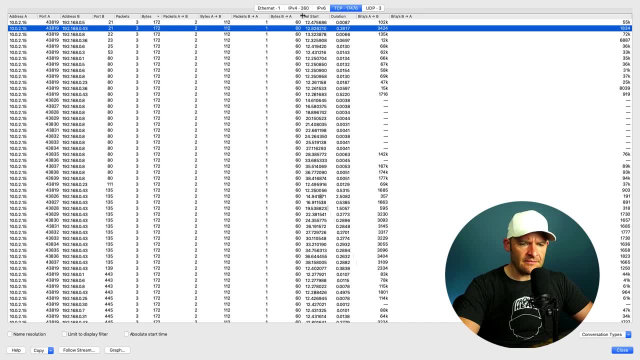 Who is 2.15? And why are they scanning through? And why are they scanning through this entire subnet looking for these open ports? Okay, so let me show you one other way that I really like to use statistics. Let me come back to the IPv4 area. 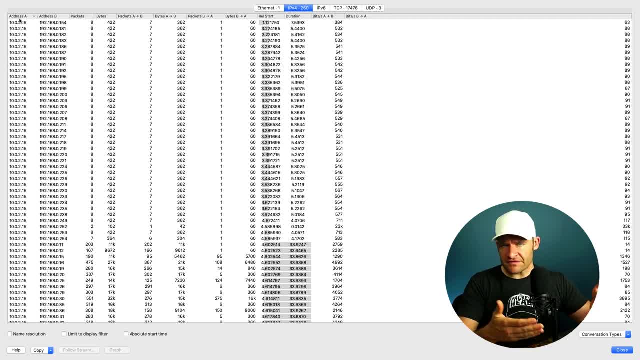 Now let's say that, instead of looking at a trace file that had a port scan on it, like we see in this trace file, what if I was tracking down a slow file transfer or some data set, a larger data set- that was moving from one machine to another? 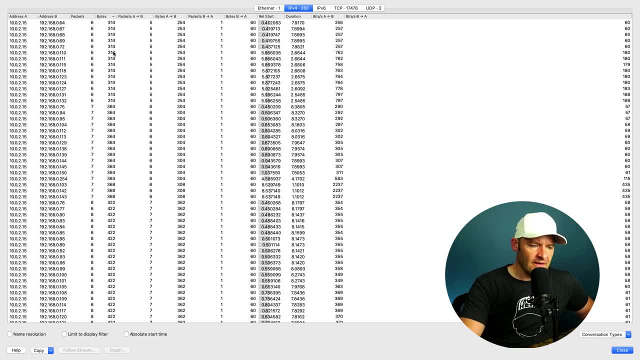 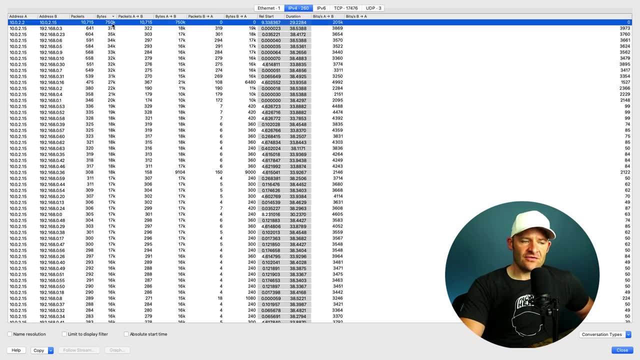 Well, an easy way to find that is if I just sort on bytes. It'll say it'll put the either on the top or bottom, depending on how I click. I can see the top talker, the chatterbox, the chatterbox conversation between those two endpoints. 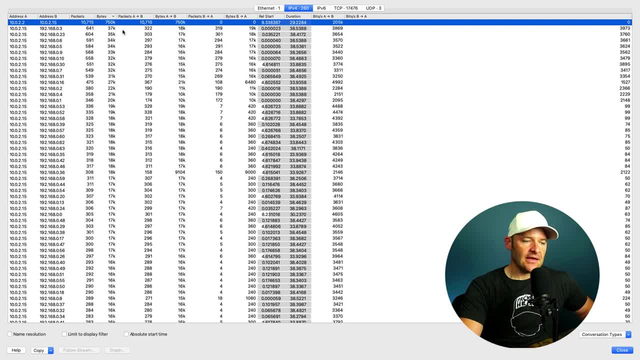 It will rise to the top or it'll be at the bottom, depending on how I click Now. often, what I'll do is I'll use this just to see, okay, who's talking to who and which conversation am I really looking to analyze? 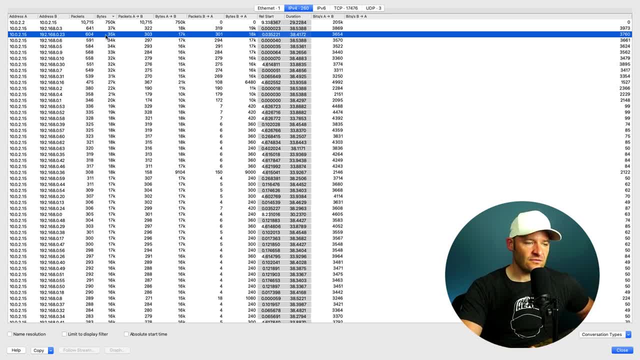 From here. super nice that we can do this. I just right click apply as filter selected And likely. what I'm looking at is the data set, And現在 iseх я ailое рассчитываю is a to b and b to a bi-directional traffic between those two stations. 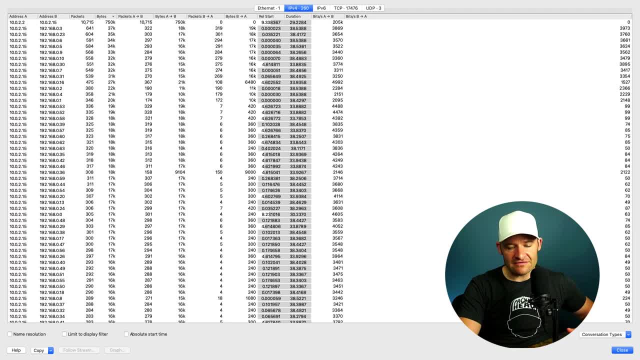 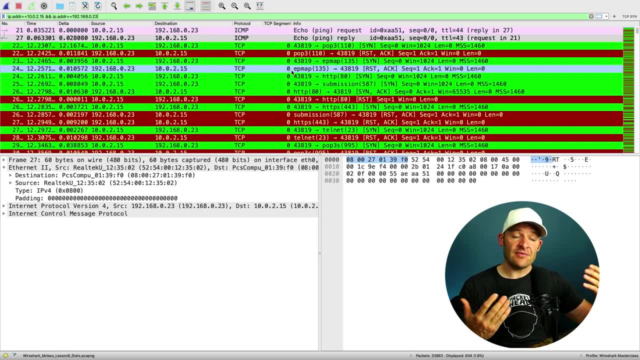 All right. So as soon as I click this Now I can say close, and Wire Shark will have filtered on those two endpoints. Now the nice thing about doing it from the IP level. Well, here I can see I have both ICMP.